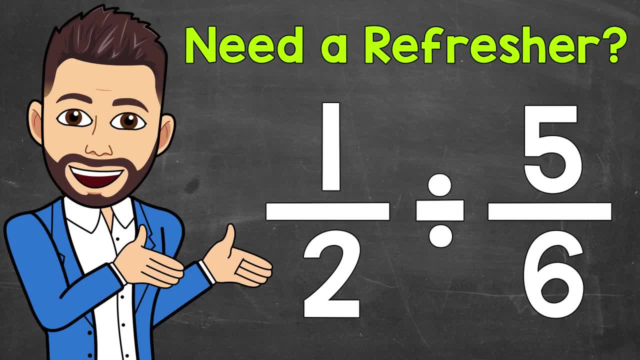 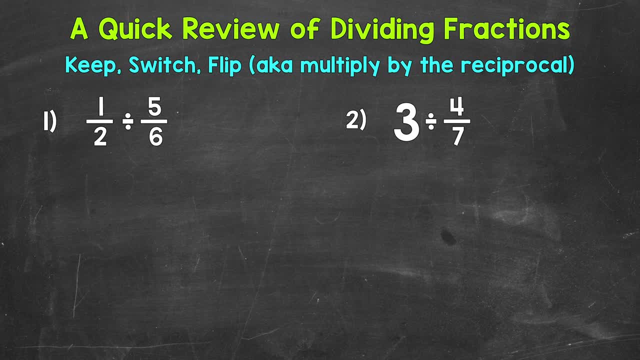 Welcome to Math with Mr J. In this video, I'm going to go through a quick review of dividing fractions. If it's been a while and you need a quick refresher, this should be helpful Whether you're in middle school, high school, college, continuing your education as an adult. 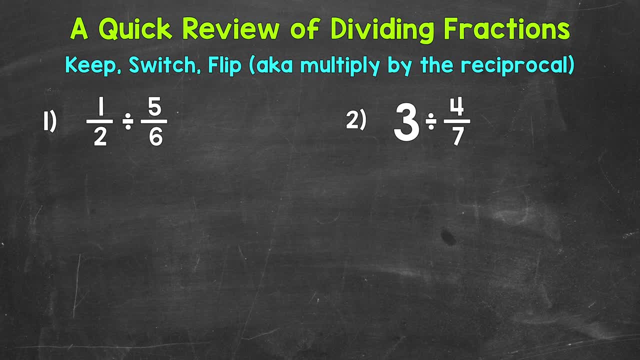 or just learned this recently. Really, no matter where you're at. here are a couple of examples to help you out. Let's jump into number one, where we have one half divided by five-sixths. Now we're going to use the steps keep, switch, flip in order to divide fractions. 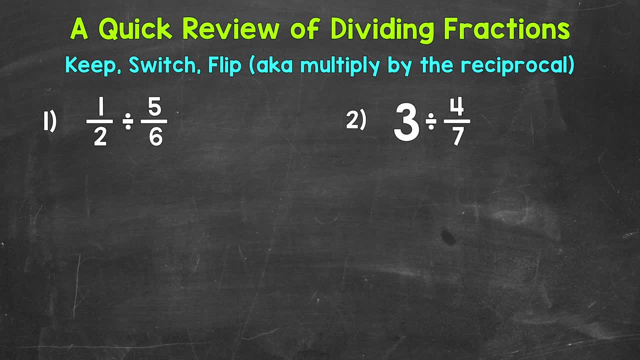 Now you may also hear: keep, change, flip, switch or change. They both mean the same thing and it's the same process. Now this is also known as multiplying by the reciprocal. So let's rewrite this problem using those steps and see exactly. 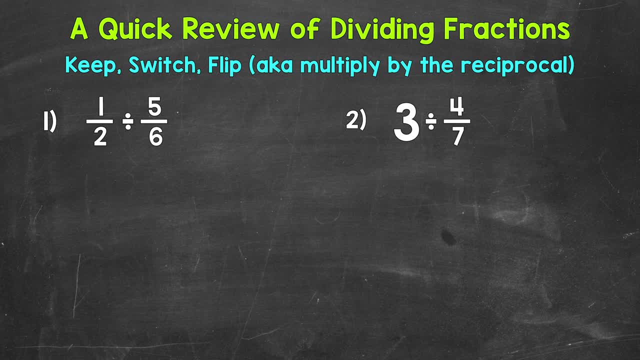 what we're going to get out of this. So we always keep whatever comes first. So we have one half, So let's rewrite one half underneath. We keep, Then we switch or change to the opposite of division, which is multiplication. 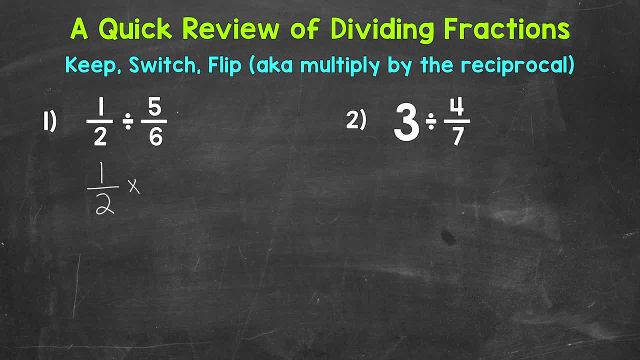 So let's write a multiplication sign And then for our second fraction we flip that fraction. That's called the reciprocal. So the bottom number, the denominator. The denominator is going to be the numerator, and the numerator is going to be the denominator. 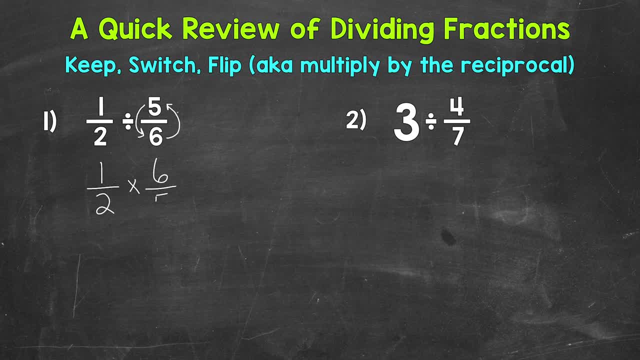 So our six goes on top and the five goes on the bottom. Now we're set up and we can multiply straight across. One times six is six. Two times five is ten, So we get six-tenths. 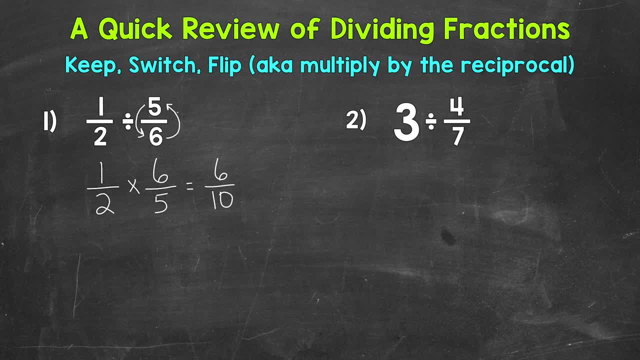 Now, six-tenths is our answer here, But we can also multiply by the reciprocal. We can simplify. We have a common factor other than one that we can divide both six and ten by in order to simplify, And that common factor is two. 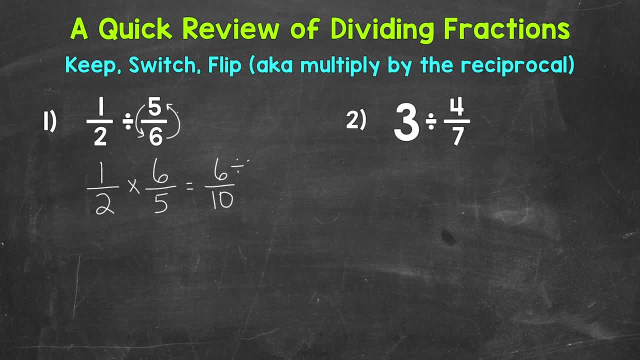 So let's divide six and ten by two here, in order to simplify: Six divided by two is three, Ten divided by two is five. So our final simplified answer is three-fifths. So again, keep switch flip. 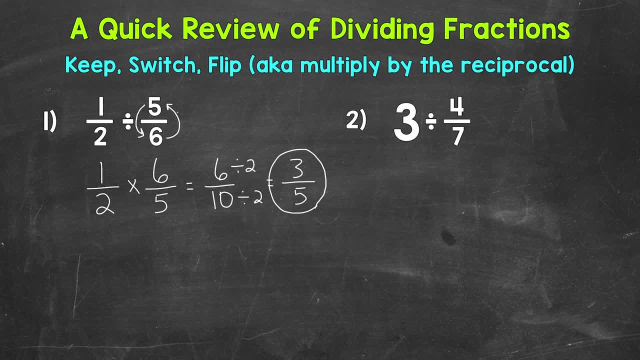 Then we can multiply straight across and then look to simplify if necessary. Let's move on to number two, where we have three divided by four-sevenths. So keep switch flip. Now we have a whole number here and we need to rewrite that as a fraction when we keep it. 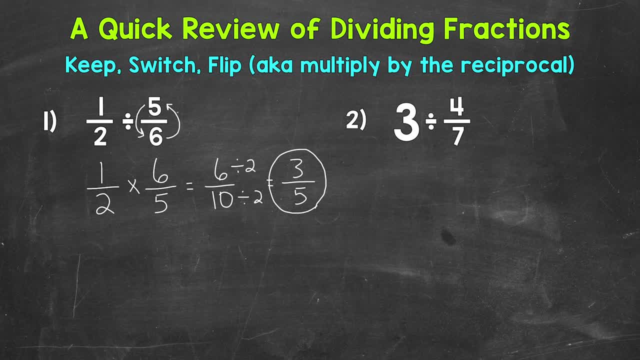 And we do that by putting it over one, And it's as simple as that. So three Over one, That still has a value of three wholes. Again, it's just in fractional form. That way we have a top and a bottom and we can go through our steps. 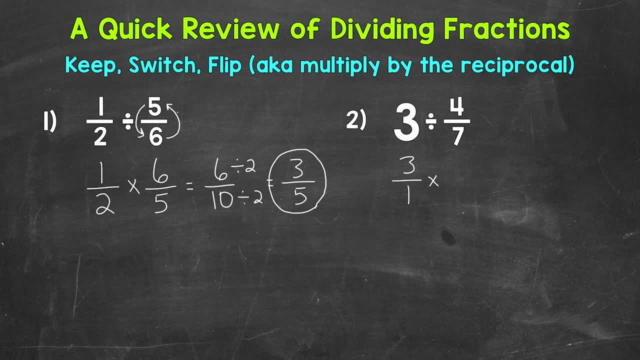 Then we switch or change And then with the second fraction we flip. So the seven is our numerator and the four is our denominator. So seven up top, Four below. Now we can multiply straight across Three times seven. 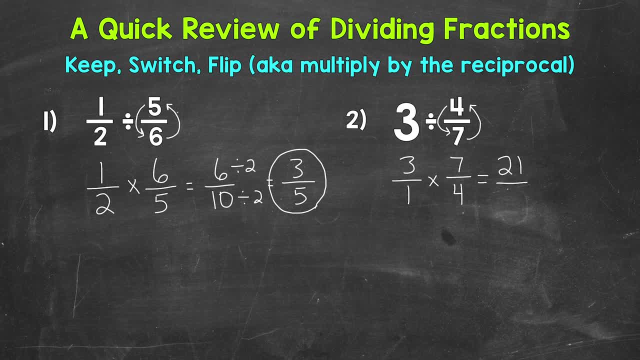 Twenty-one, And then one times four is four, So we get twenty-one-fourths, which is our answer, but it's in the form of an improper fraction. So let's convert this to a mixed number, And we do this by dividing our numerator twenty-one by the denominator four. 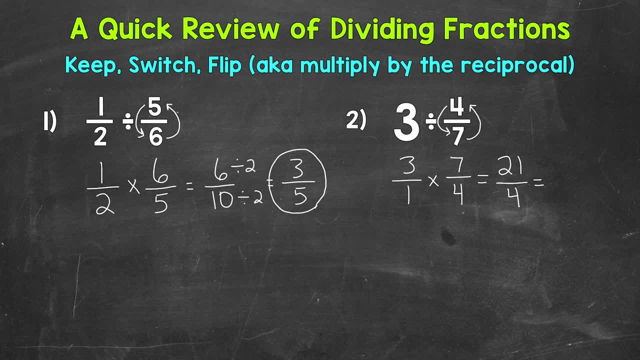 So this is going to equal: How many whole groups of four can we pull out of twenty-one? Well, five whole groups of four. That gets us to twenty. We have a remainder of one. That's our numerator, And then our denominator of four stays the same. 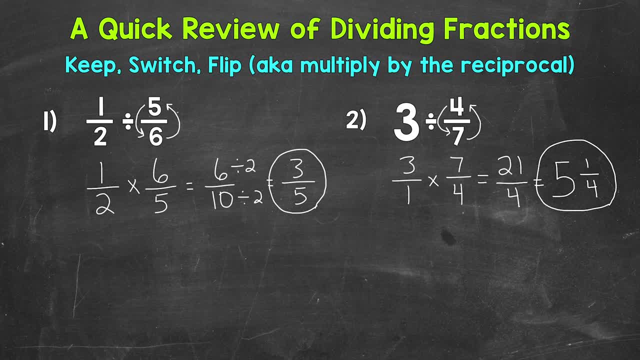 So we get five and one-fourth. Now let me go through how I converted that improper fraction to a mixed number. one more time I'm going to write it. So we do twenty-one divided by four. So how many whole groups of four in twenty-one? 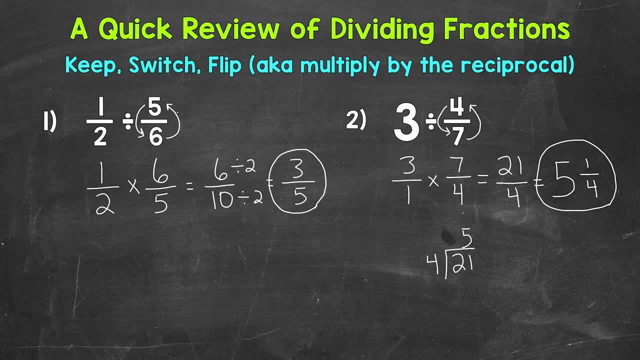 Well, five, That gets us to twenty. Five times four is twenty Subtract, We get a remainder of one. So this five is our whole number, Five whole groups of four in twenty-one, And then our remainder of one is the numerator of our fraction.